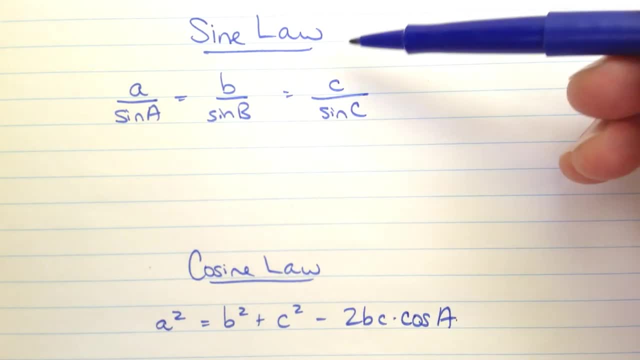 Hi, I'm Brandon Graceland. I'm a high school math teacher. Let's look at sine law and cosine law and when you should use each one to solve for part of a triangle, Here's the sine law written with the length divided by the sine of the opposite angle: A over sine. A is equal. 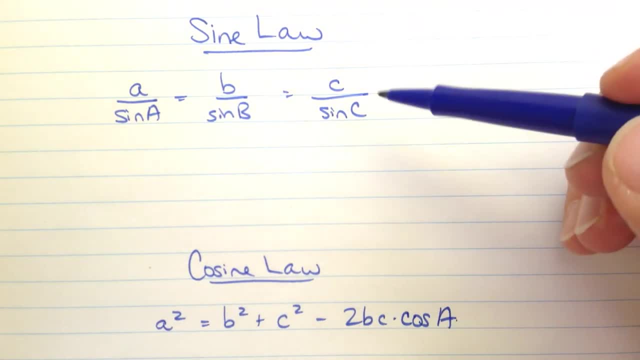 to B over sine B, which is equal to C over sine C, And you can flip this over. the reciprocal of this: sine A over A equals sine B over B, equals sine C over C, And so, to use this, you've got to know three out of four pieces of information from two of these ratios. So 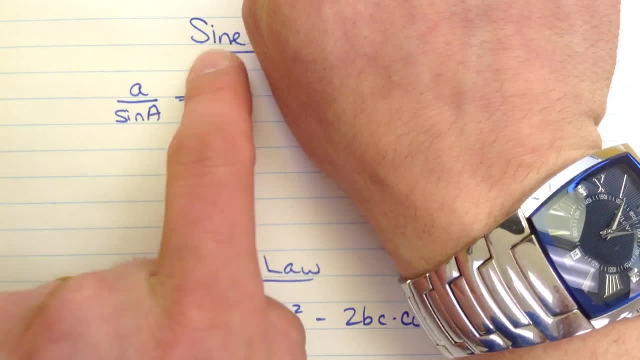 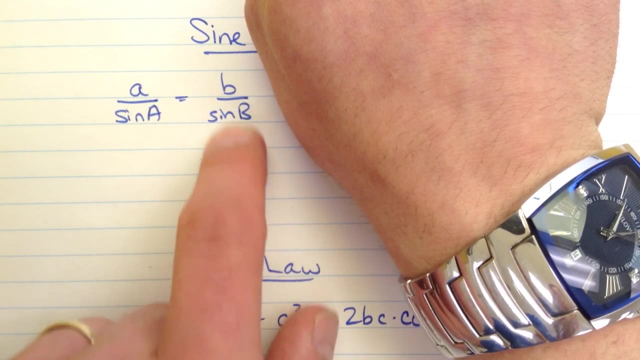 for example, you might know little, a little b, capital A, the angle, but you don't know capital B, And so if you fill in the other three values, you can solve for the remaining value. That's great, as long as you know three pieces of information from any two of the. 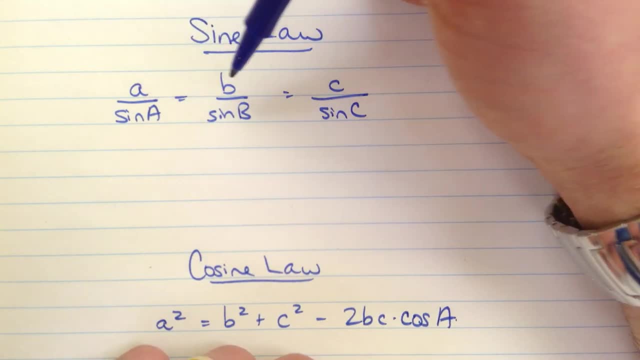 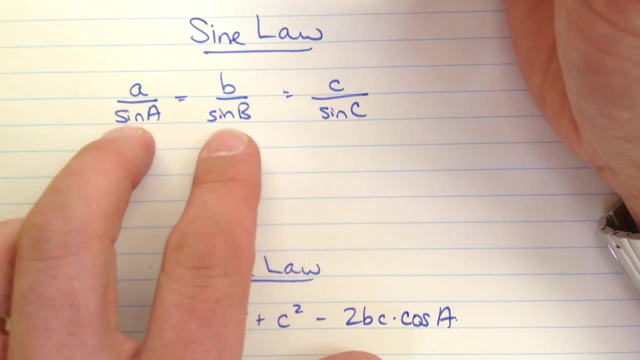 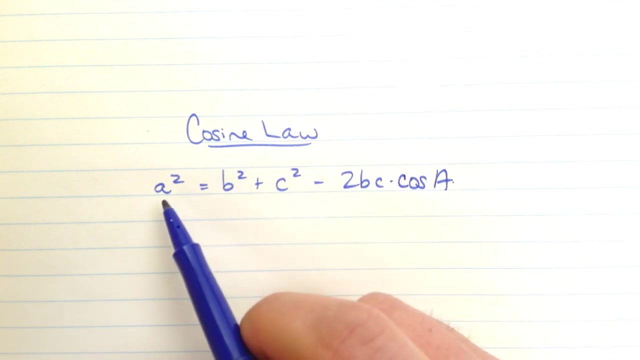 ratios. But, for example, if you know A, B and angle C, that's not helpful because you have three separate parts to this. You would need to know at least one of these angles, or you would need to know side C. But then we have the cosine law. This has three sides. All three sides are written. 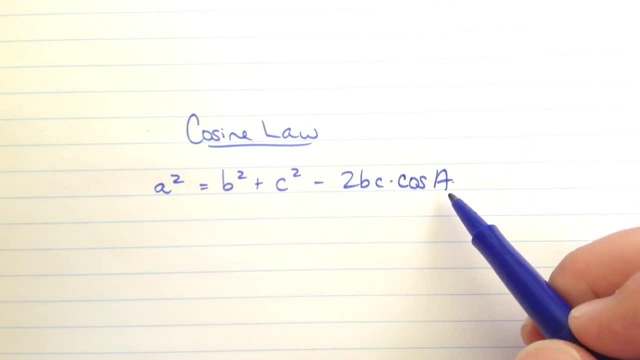 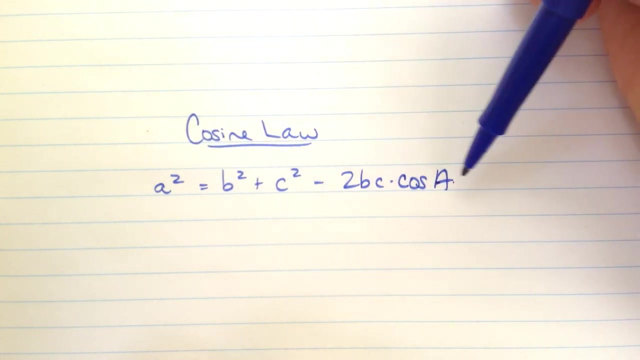 in here A, B and C and one angle, And you can reorder this and switch around which sides and angles you have, depending on where you're sort of standing on the triangle, which angle you want to find or which angle you know. And so, if you know, again, there's four pieces. 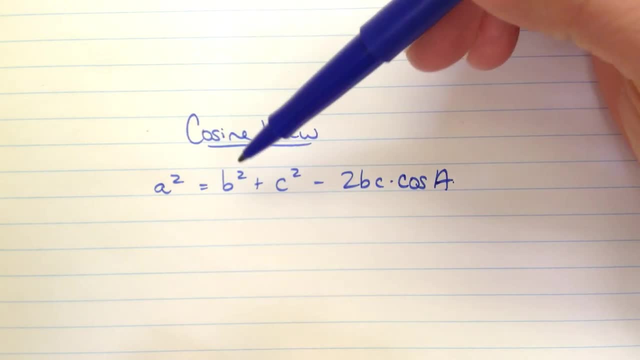 of information, three sides and an angle. If you know the right pieces, three of those pieces of information, you can find the remaining missing item. So, for example, if you knew all three sides, you could find the remaining angle. Or if you knew the angle A and you 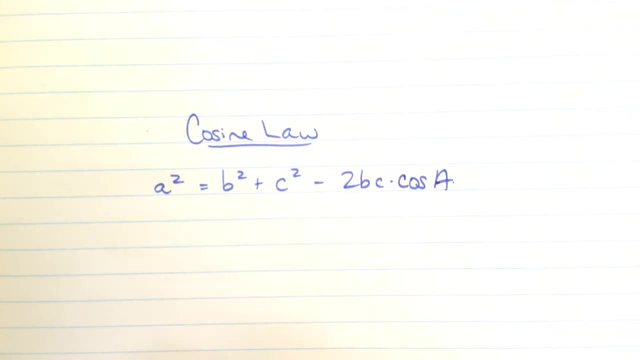 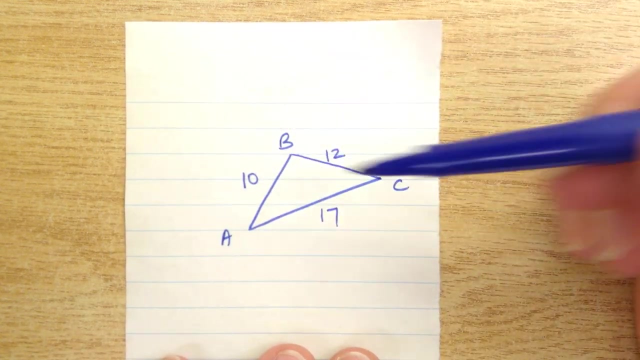 knew B and C, you could find little a. Okay, so let's look at some examples of the different kinds. Here's a triangle with three sides, that we know. We don't know any angles. So you can see then that the sine law is not. 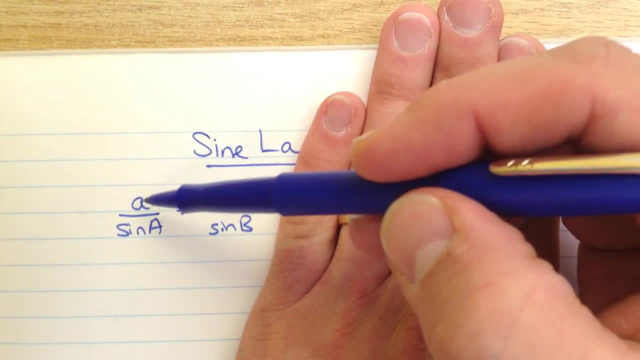 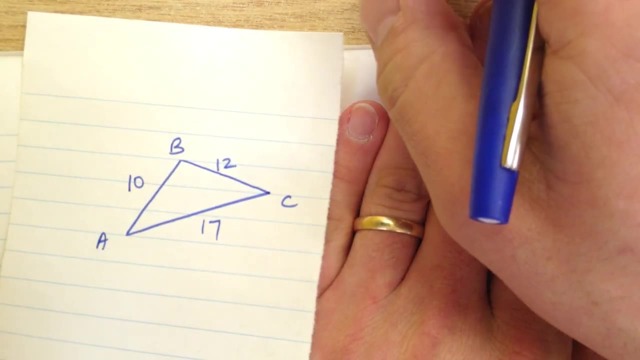 going to be helpful for us. If I take any two ratios like these two, I'm going to need three of the four pieces of information Here. I know A and I know B, but I don't know any angles, So I can't fill in this and I can't fill in this. Sine law is no good for us. 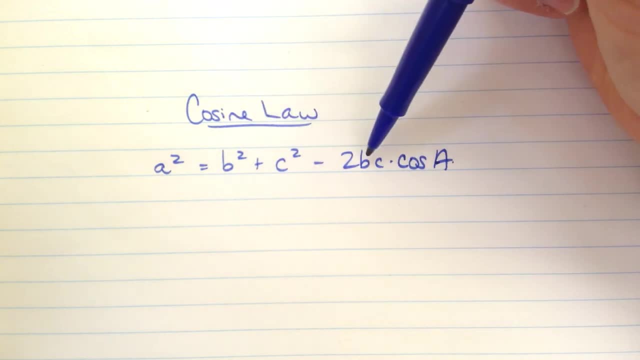 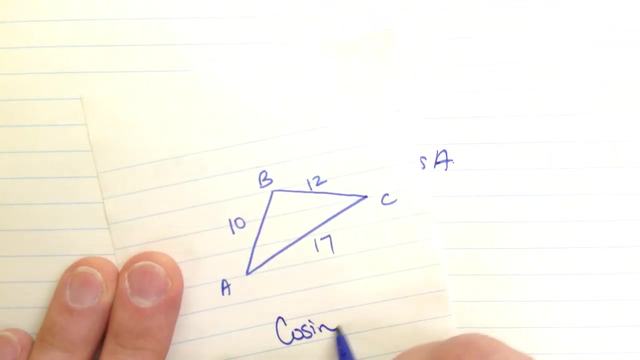 But cosine law is: I can fill in this, this, this, this, this- I just don't know this- angle A, So I can fill in the rest of it and solve for A using my inverse cosine function. So that one is cosine And we often will write down a little abbreviation because this one 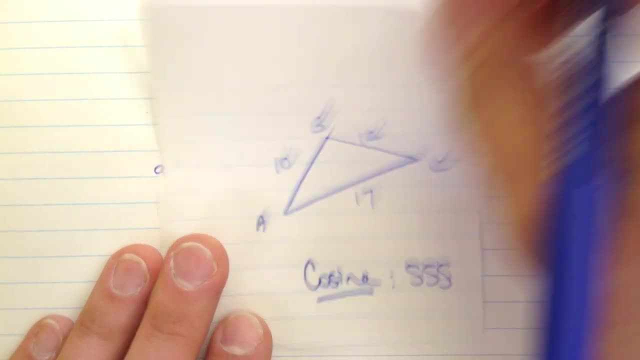 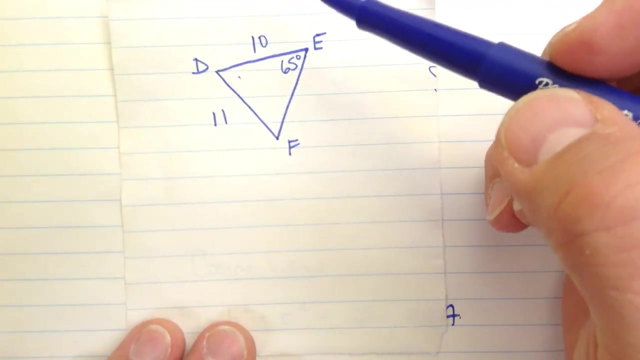 is side, side, side. We have three sides. We get to use the cosine law. All right, let's try another one here. How about this one? D, E, F? here I've got two sides and I have an angle. Now I'm being careful, though That angle is over. here I've got 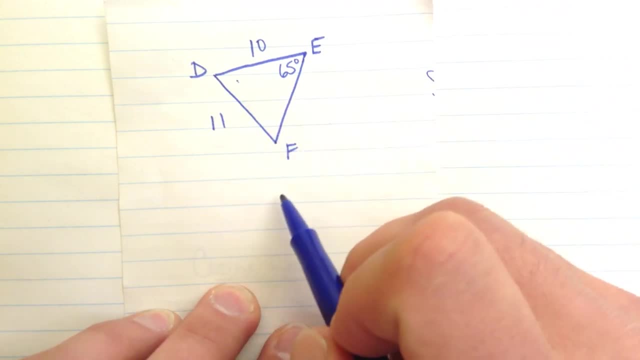 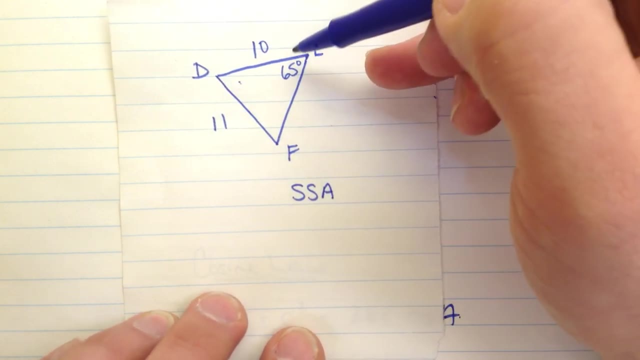 two sides and the angle is not between them. So we might write- we often write side side angle because the angle is not between those two sides. It's important To solve this. I have an angle and the side across from it and one more side That looks to me like sine. 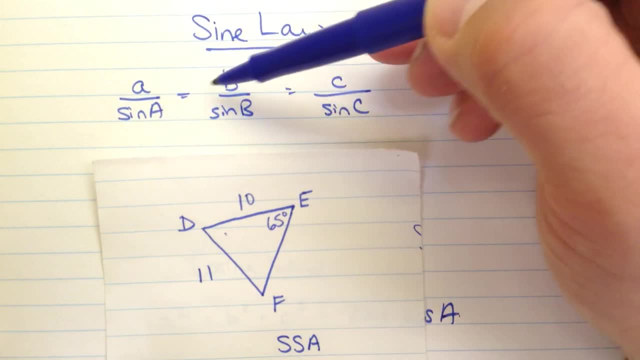 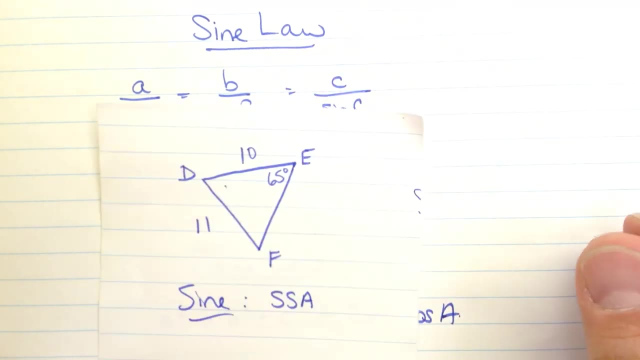 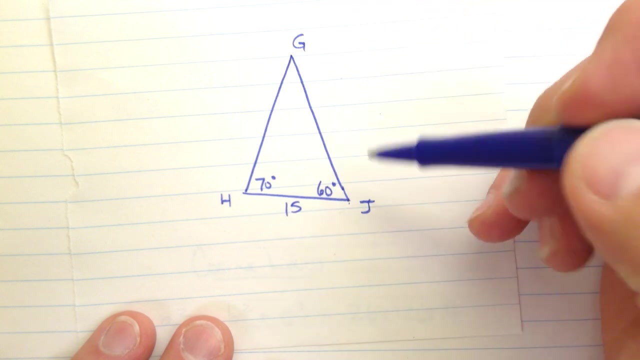 law. I've got two sides and one of the angles that's across from one of those two sides, So I just have to find the other angle. That one is sine law. Nice, How about this guy? Triangle GHJ? I avoided the I because it looks like a. 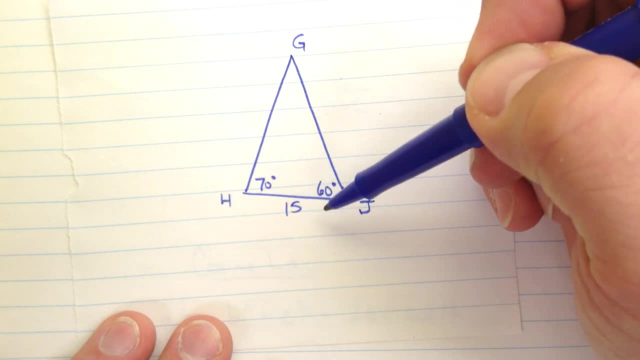 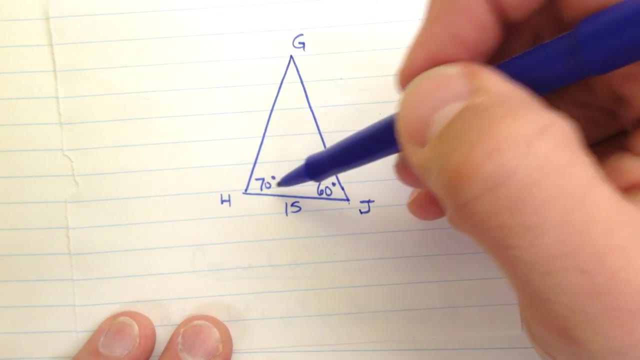 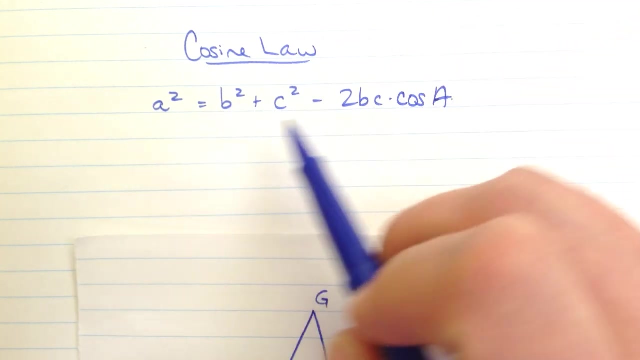 one. I have two angles and I have a side. Well, let's see here. I can't really use cosine law here because I have two angles and only one side. The cosine law only involves a single angle, and I have to at least know two of the three sides to be able to use it. So that's. 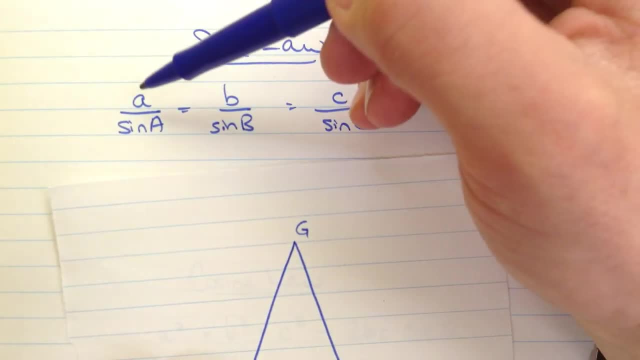 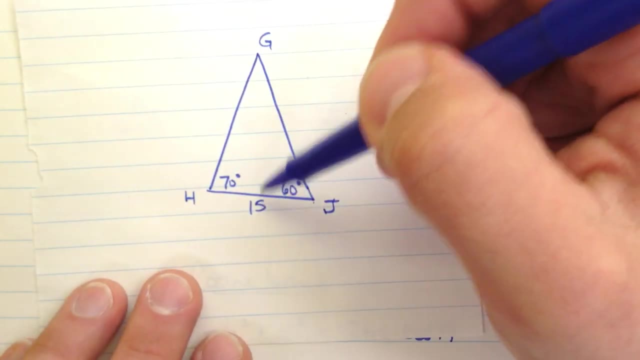 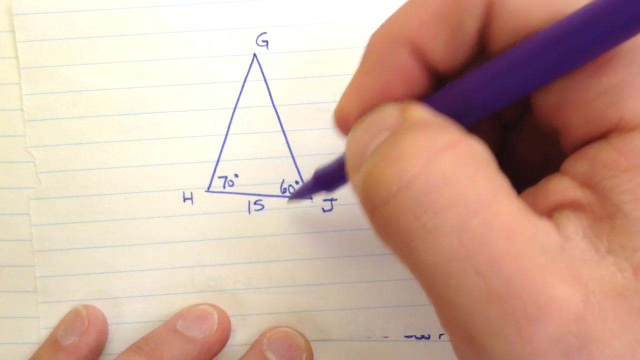 no good, But I can use the sine law right, Because I have, let's see, I have one side, I can find the other side if I know the angle across from it. Well, I don't, OK, OK, angle across from this, but I can figure it out, because 70 and 60, that adds up to 130 the whole.